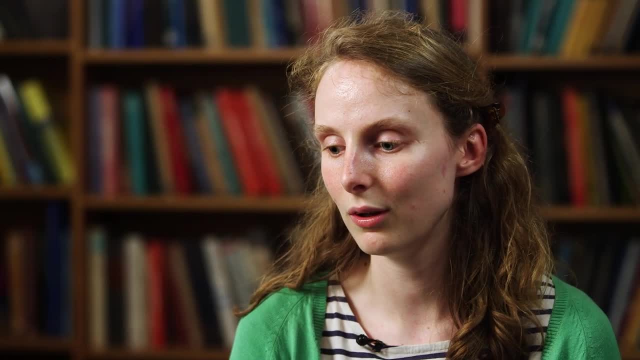 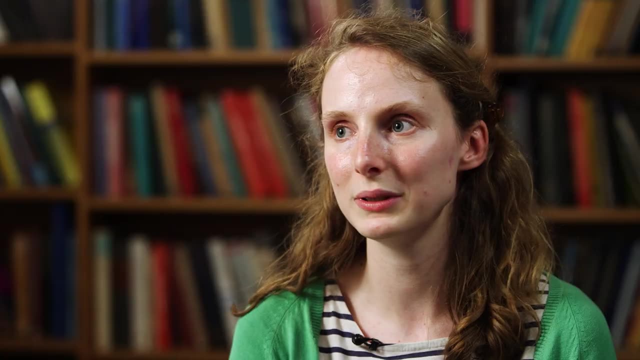 It's difficult, not really knowing what to do. You will get stuck. you will feel frustrated. You've got to understand it in your own terms. No one's telling you the right way to do it. You need to be stupid so to ask stupid questions. 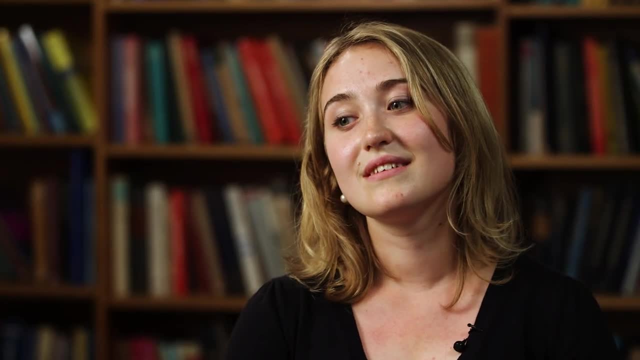 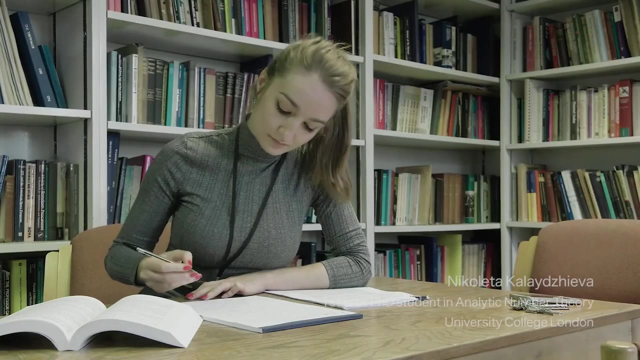 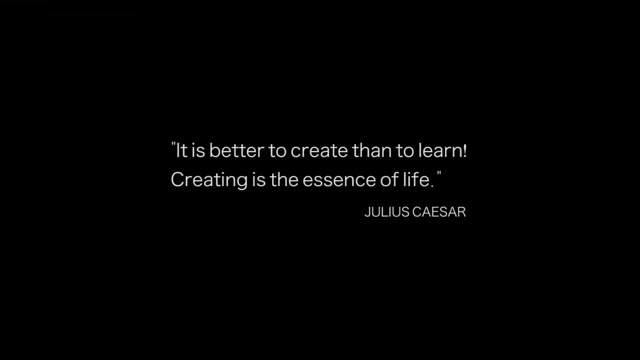 So being You need to be motivated to keep asking the questions. And then that moment when it clicks, or when you finally solve something, it's this rush of enthusiasm and excitement, Huge relief and joy. The results arise so naturally inside us. 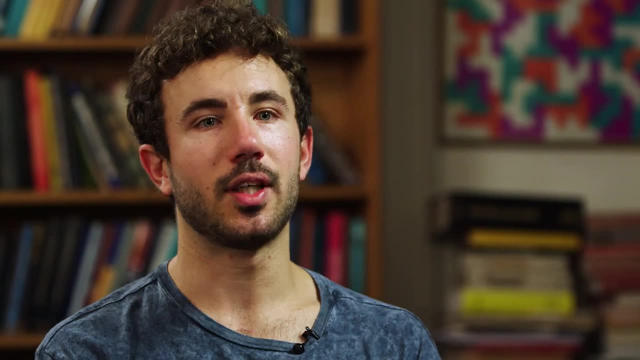 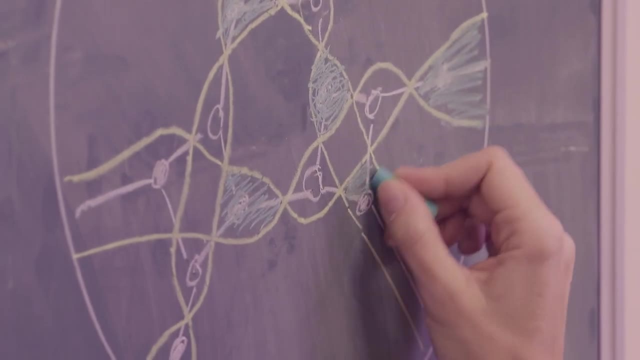 It's like they're already there And they're just waiting for us. It's not that it's all in your head, but it's a much more inventive and artistic time. You have these unwritten rules about beauty and elegance and trying to get where you want. 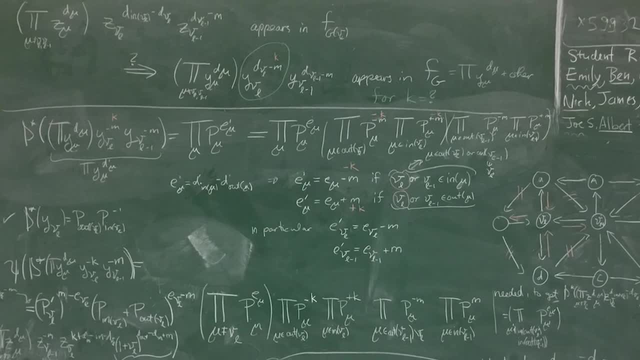 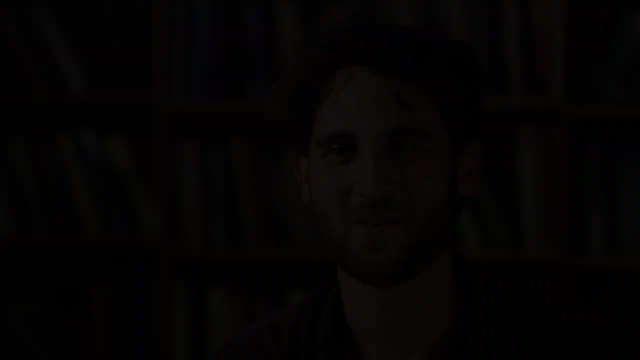 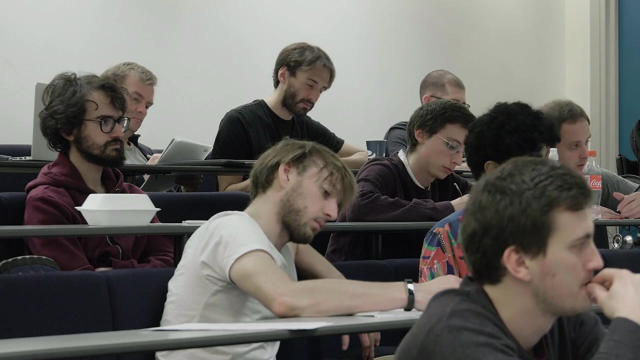 to be in the nicest way possible And these rules are a bit vague. but still, most people, if they see a beautiful proof, most people will agree: yeah, that's very beautiful. The program is structured in a way that lets you find out what you really like, what you. 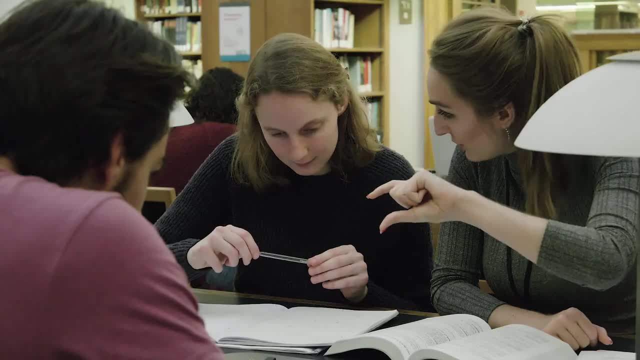 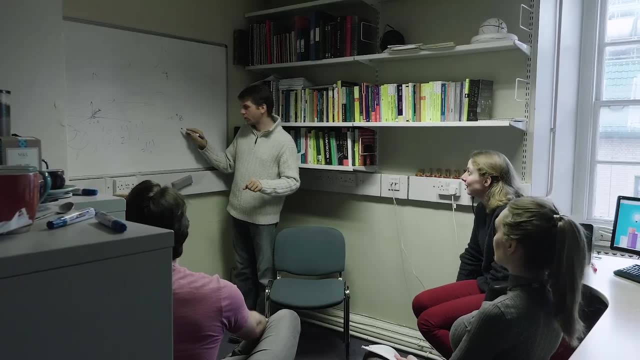 really want to do. You're no longer being told what to learn. I really like this. I really like that the first year had lots of courses and that you got to pick your supervisor. at the end, You can try out different supervisors. I think that's incredibly valuable. 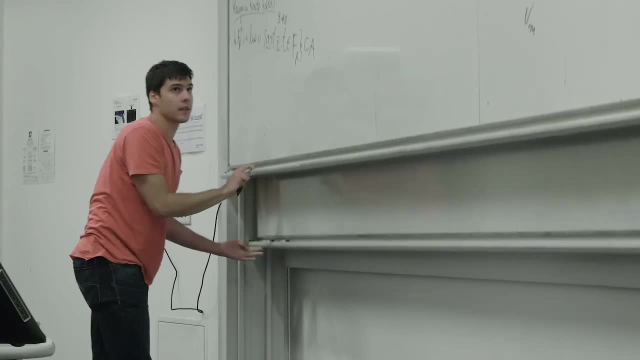 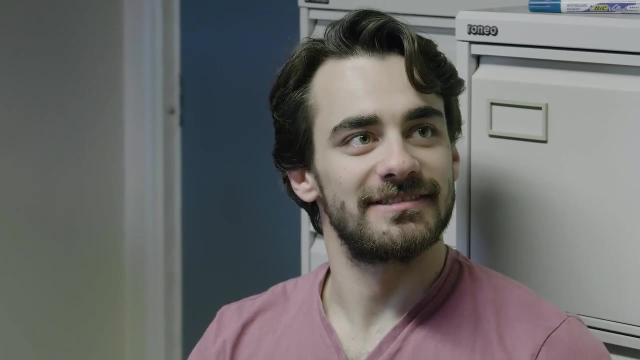 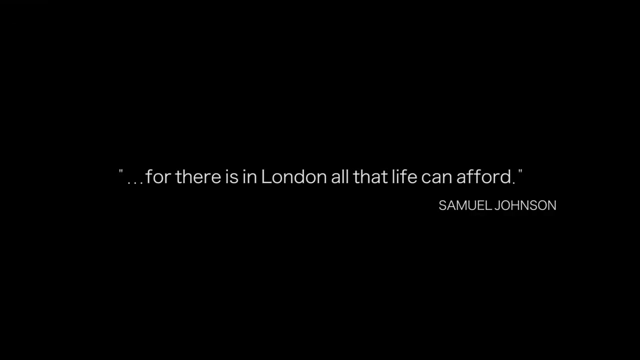 You kind of get bombarded with new ideas every week. You're looking at things in a broader way, but you're also specializing and looking. So you're looking at one very specific thing, but with as many tools as you have, And it was four years as opposed to three. 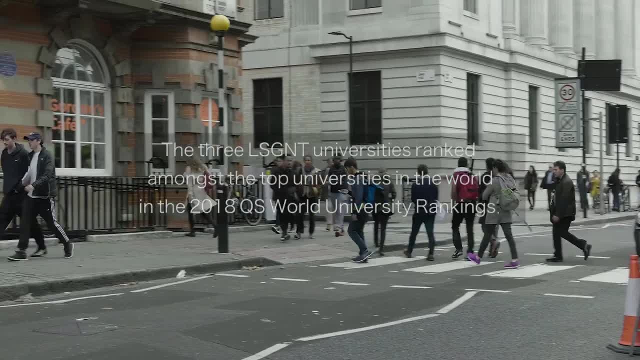 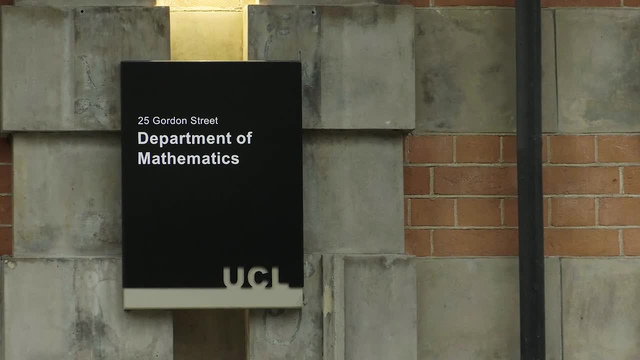 London Astaire is one of the few European cities that has different, very good universities. You're really a PhD student of all three universities for the entire four years. These three universities is that, for instance, for number theory and geometry, they collaborate. 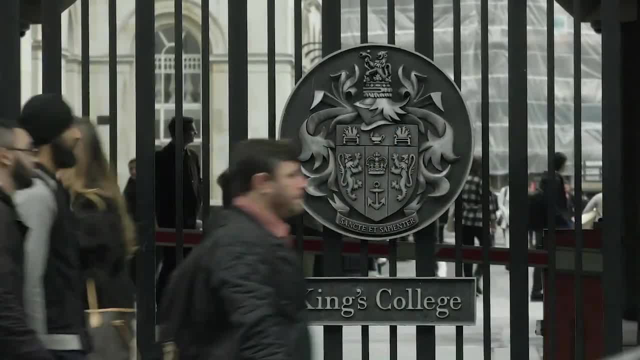 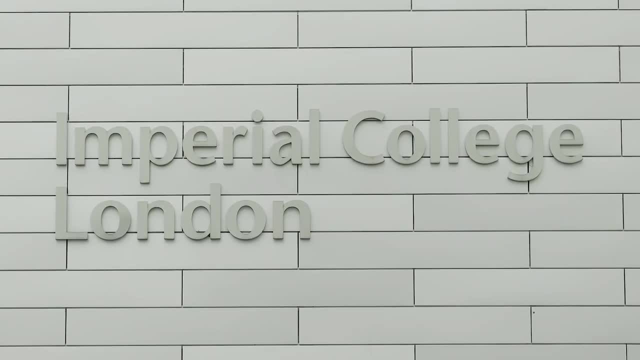 all together, You can choose supervisors at three universities, and there are a lot of people, for example in the year above us, who have one supervisor at one university, one supervisor at another university. They spend different days in different places. They're exposed, therefore, to a wider range of supervisors. 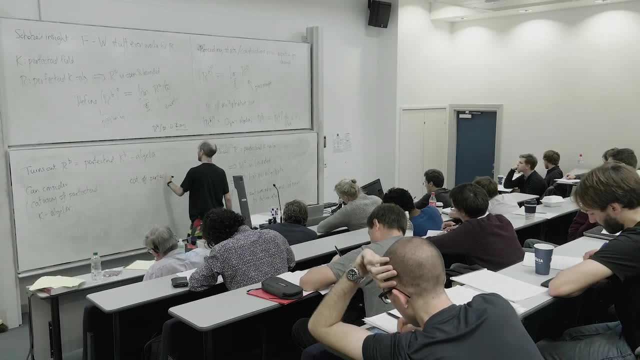 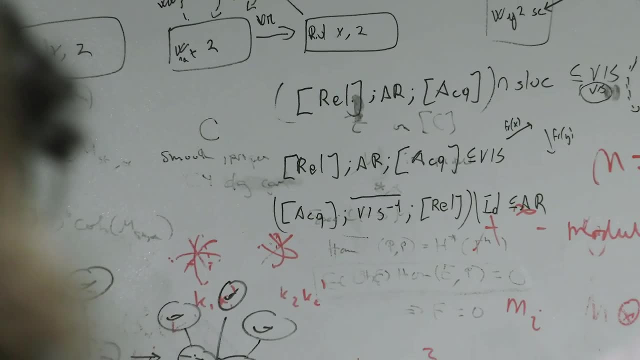 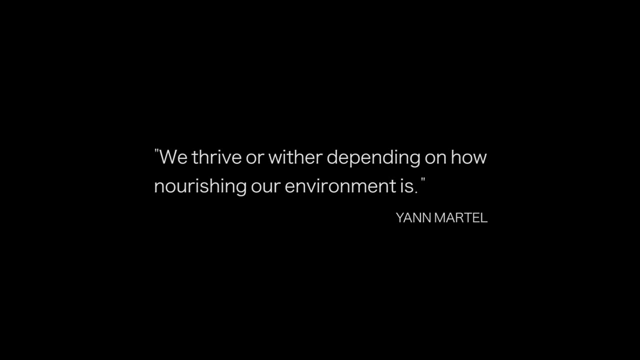 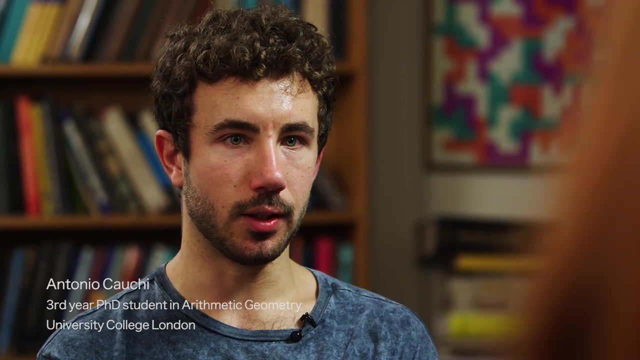 London Provincial University. It probably has more geometers than any other city, at least in the UK. It's an incredibly active place to be and there's tons of seminars going on. It's really, really a great place to be. This is one of the things that I most liked of the LHGT program. 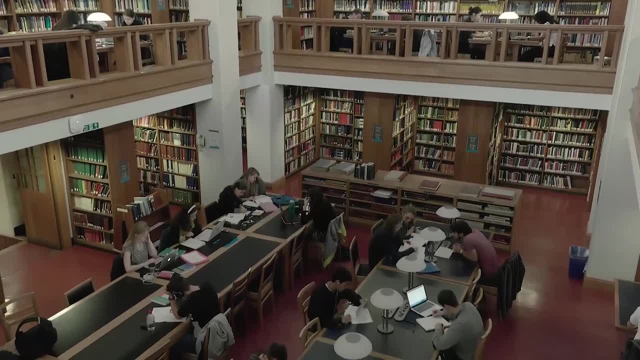 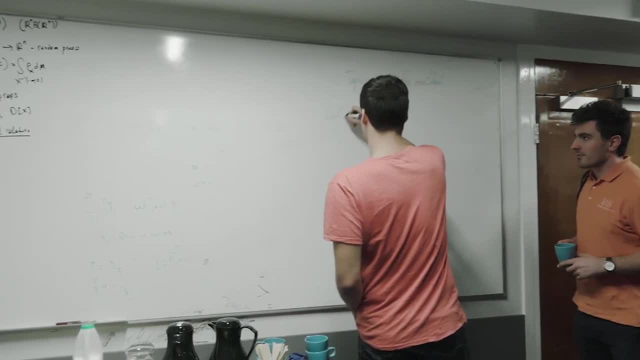 If you had a problem, you had a lot of people to talk with. We all discussed things amongst us, So everybody knows a bit more about a particular field, so you get to see a bit more. There are so many students coming together to the same place and so they talk to each. 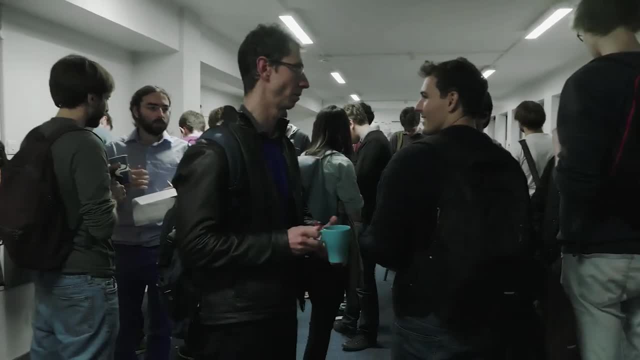 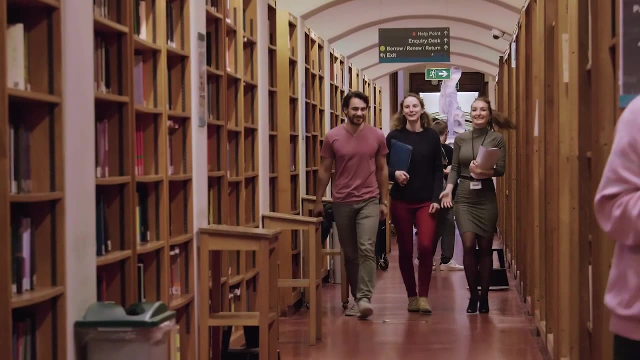 other. they explain things to each other. they all come with different backgrounds. I think it can be very isolating to do a PhD in some places where no one else knows anything about what you're doing. I was kind of aware of how good that collaborative aspect would be before I came. 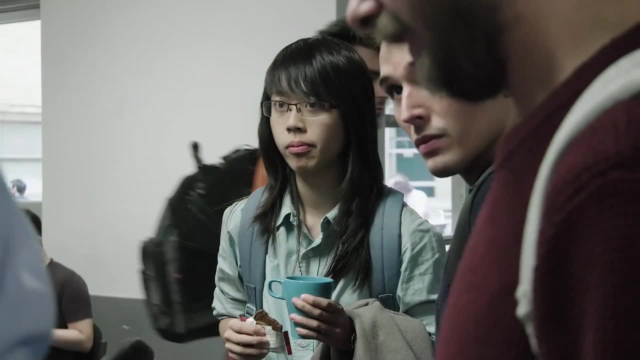 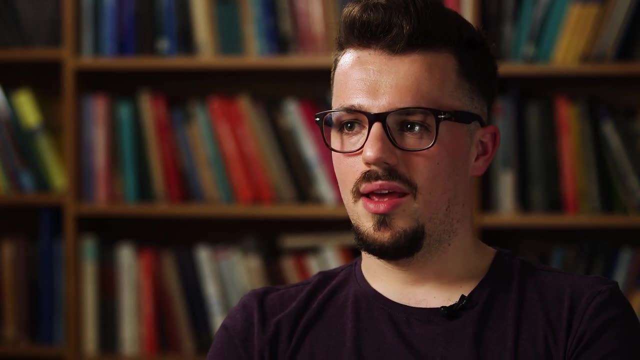 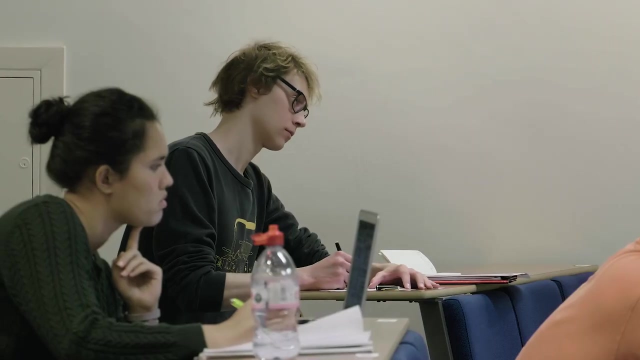 It's also really enjoyable the fact that you can talk about your passion. It's really fun. It's really fun, It's a wonderful passion, and the fact that your passion is your job. it's a wonderful mix. So, all through being an undergrad, you are paying to go to university and have someone. 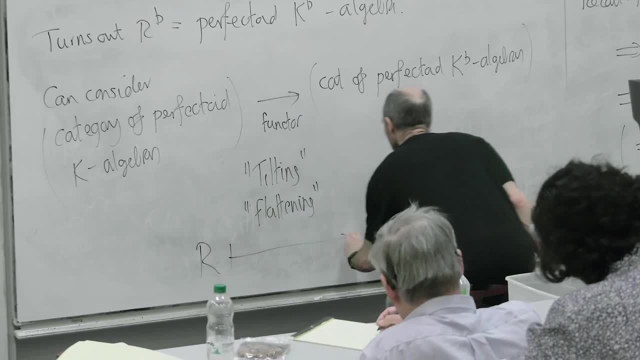 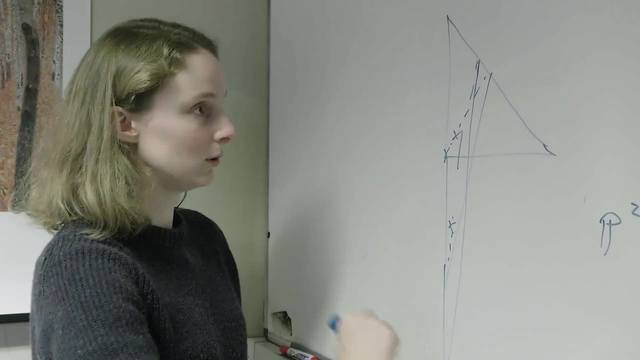 teach you maths and you're paying to go there and have them teach you what maths they want, And then suddenly it's like a huge paradigm shift because they start paying you and you can choose the maths. So it's like both aspects get way better. 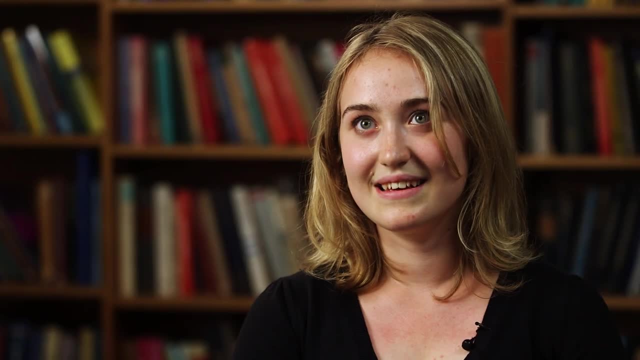 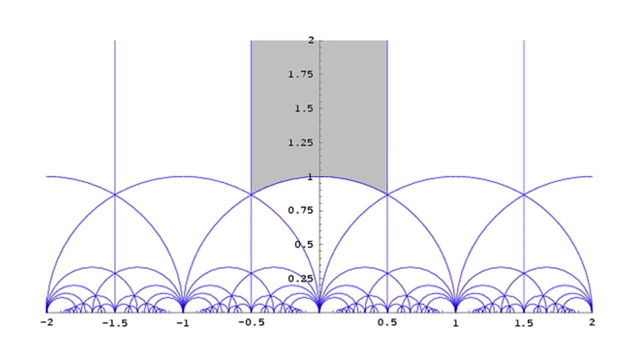 A big part of the beauty is the support. Yeah, For me at least, is the surprising otherness about it. You have to learn this language before you can appreciate the beauty properly. Once you do, it's the same kind of beauty as is in music and other things like that. 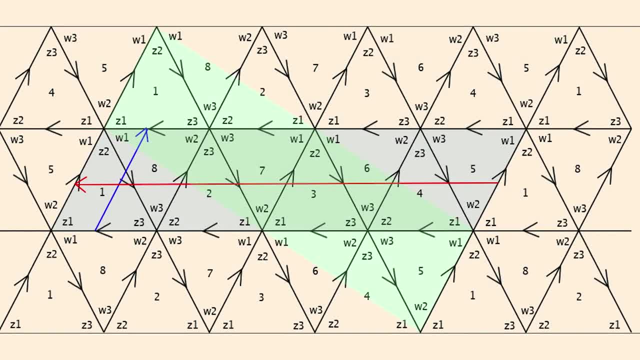 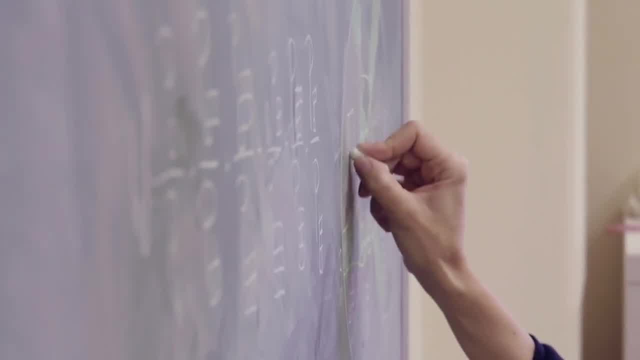 If you're like a visual artist and you look at paintings all the time. the more you look at them, the more structure you see and the more beauty you detect in a painting like that, and maths is like that. It's how the nature communicates with us.